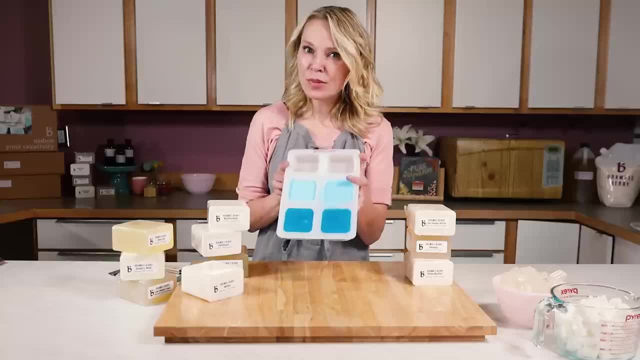 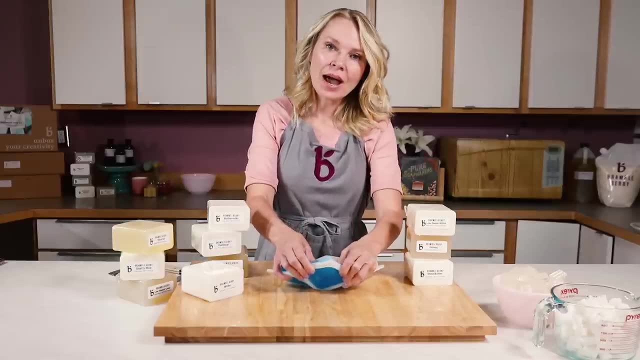 rinse away cleanly and leave your skin feeling great when done So. keep in mind that a clear base gives you more saturated colors and a white base gives you more pastel colors, And this is because, when you add color to clear base, it's not competing with anything, right, you just have the 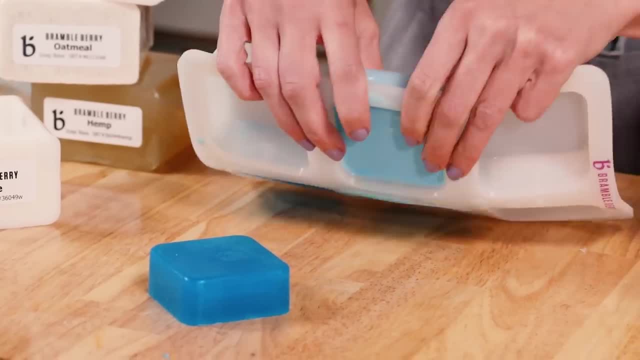 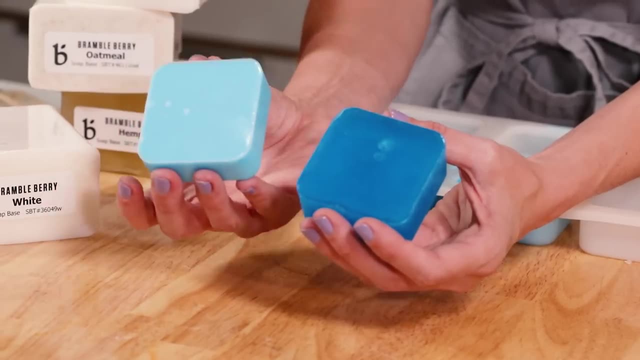 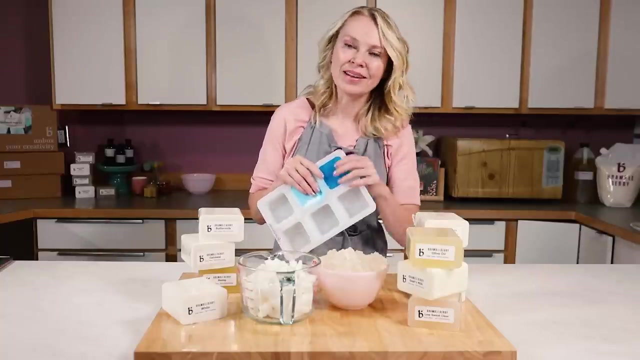 clear plus the color, whereas when you add color to white base you're basically making a pastel right. you're adding white and colors together and so you get the pastel look versus the kind of brighter, more clear look. So think about that when, like say, designing a Christmas soap with, like say, a red. 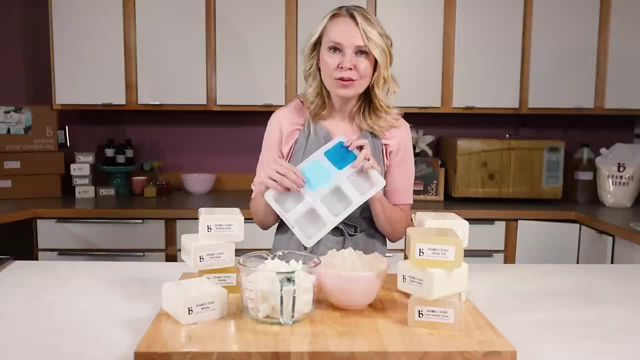 if you use white soap, you'll end up with pink. or if you're going to use white soap, you'll end up with pink. or if you're going to use white soap, you'll end up with pink. or if you're going to use black, you'll end up with gray. so if you want bright colors, that are exactly what you're. 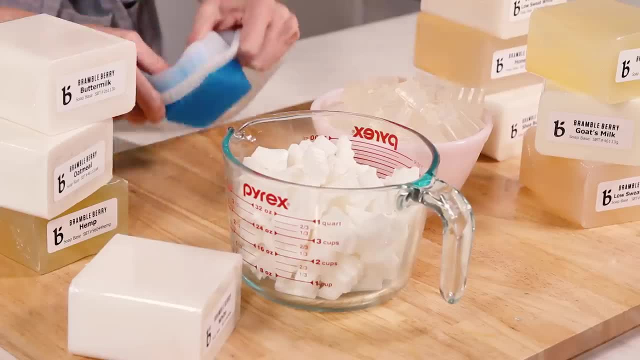 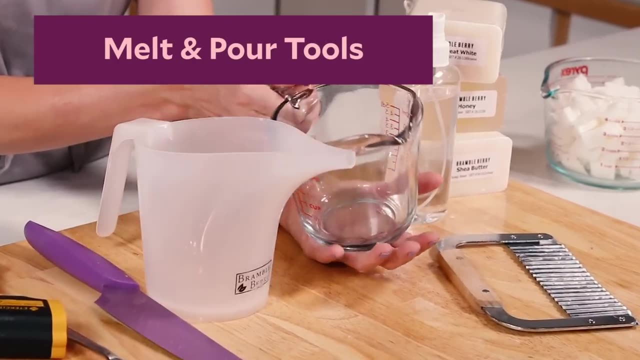 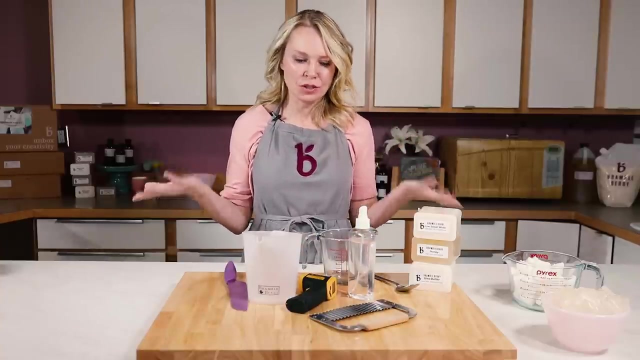 looking for color, wise, just stick with the clear soap. if a little bit of pastel is good, then go with the white soap. Another great thing about melt and pour soap is it requires minimal equipment really to get started with melt and pour soap. all you need is a heat safe container. 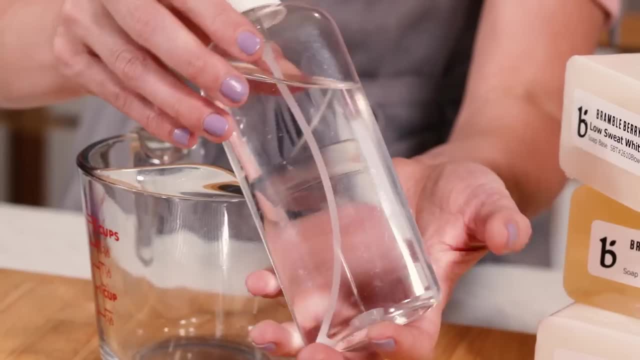 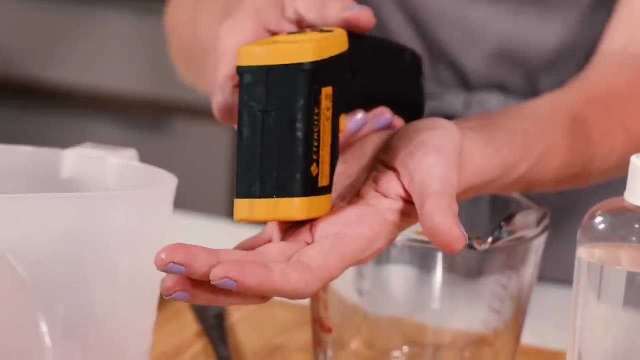 some sort of stirring utensil and optional ingredients would be like isopropyl alcohol, which help to pop bubbles after you're done pouring. maybe a thermometer, a temperature gun, just in case you want to check for layering. and, of course, your mold. now i like to use silicone molds. 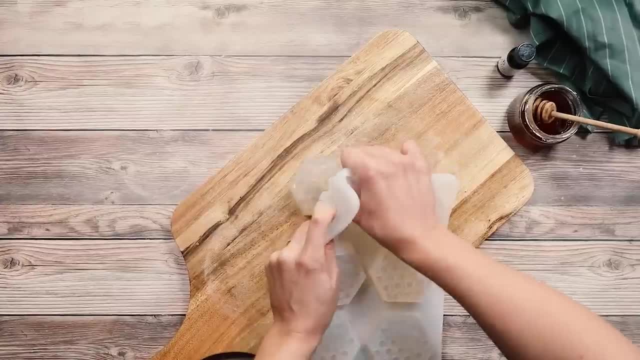 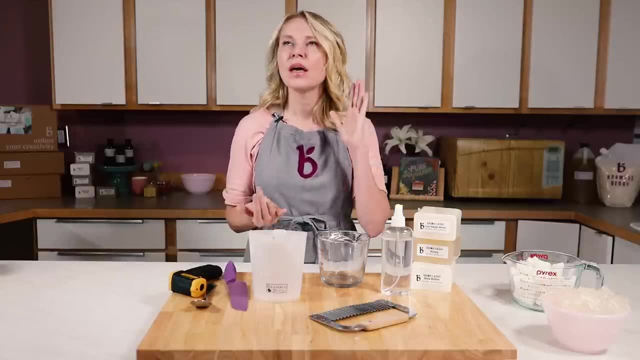 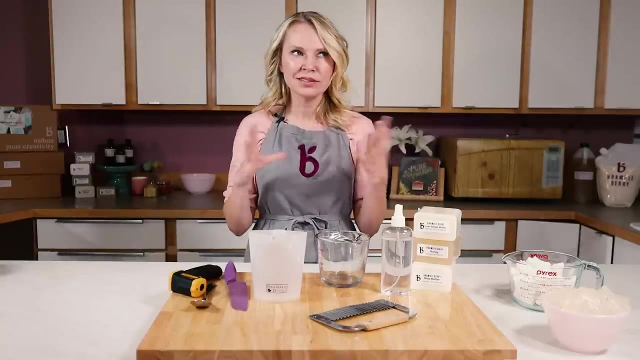 they come out really easily. they're designed for soap, but if you're just getting started, any container that has give meaning some sort of flexibility will completely work for your soap making process. so think like cleaned out tofu containers or yogurt containers or tupperware. definitely never use metal or glass, though, because you'll never get that soap out. 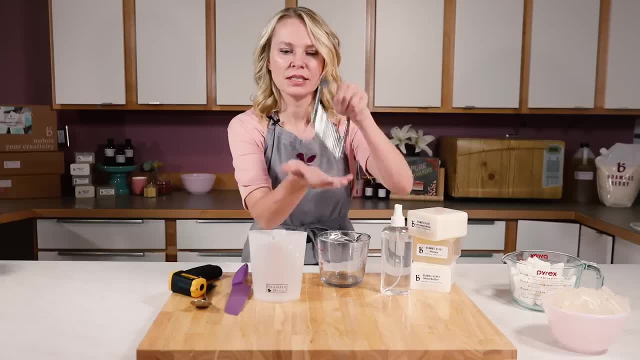 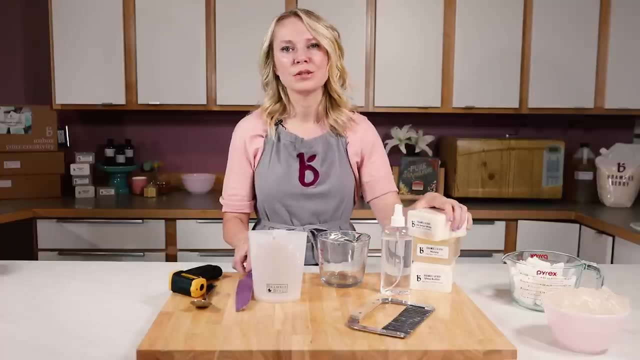 you need is, of course, some sort of cutting utensil. so i like to use this crinkle cutter from brambleberry. it's nice and sharp and it cuts cleanly through the soap. but if you have a regular knife at home, you can absolutely use just any regular kitchen knife as well. 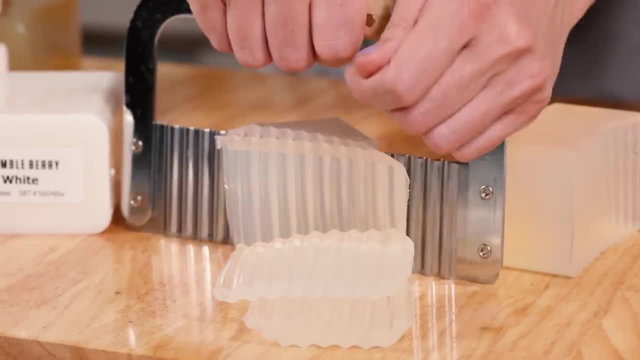 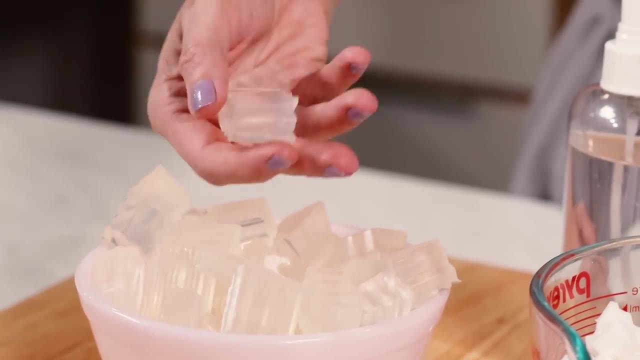 so let's talk a little bit about melting your soap, since that's such a huge part of soap making. when you're ready to start, you need to chop down a block of soap into smaller pieces, and this helps the soap melt down evenly. if i were to melt the intact, 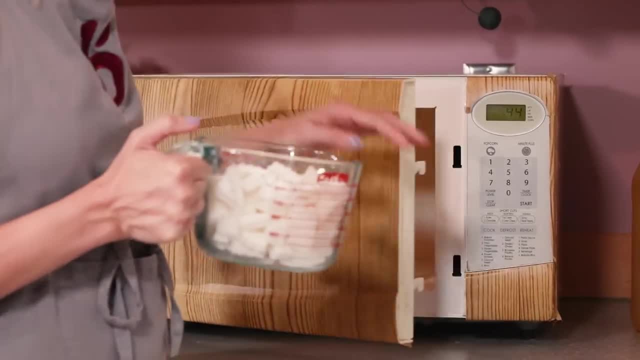 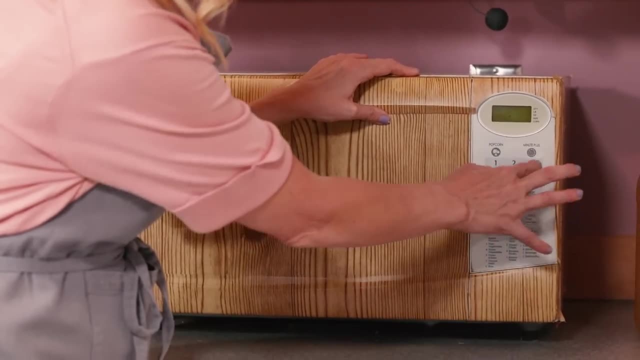 entire block, like without chopping it. some of the soap would melt quickly and become way too hot, while some of it wouldn't have melted at all. personally, i like to use a microwave to melt my soap, but you can use a double boiler if you prefer. a double boiler is especially 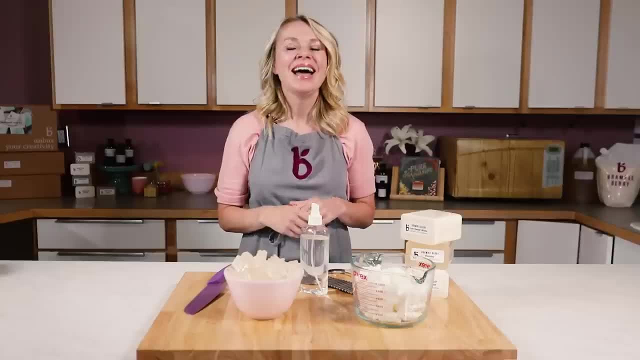 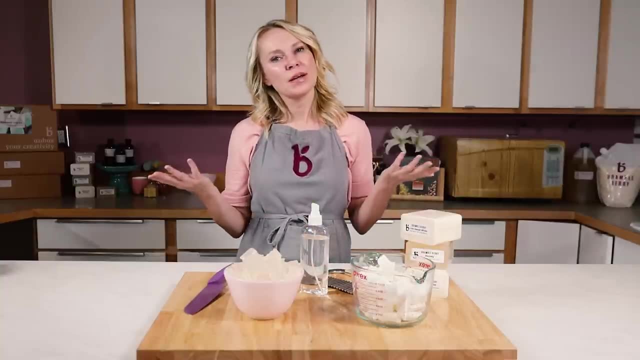 a good option if you're melting down large amounts of soap. now that my soap is fully chopped up, it's time to place it into a heat safe container and melt it in the microwave. i do 30 second bursts at a time, making sure that the soap doesn't get too hot, because the soap can scorch and burn over about. 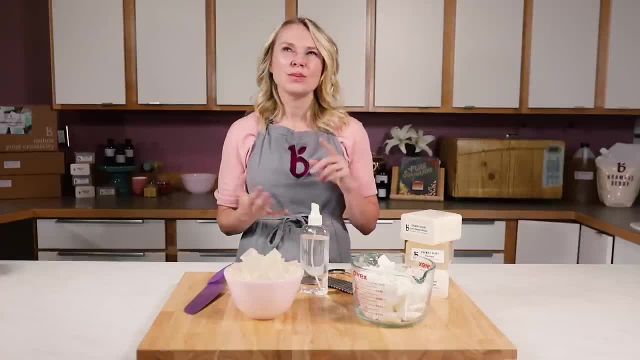 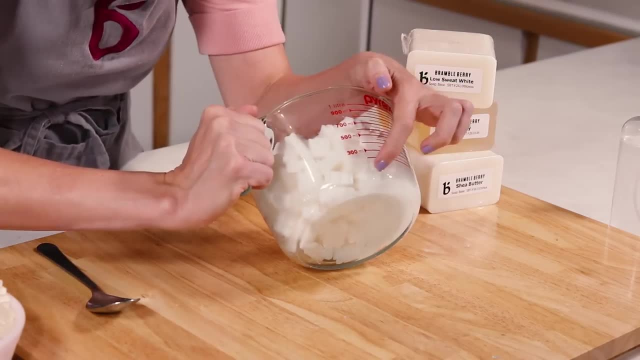 and when that happens it turns an extra yellowy color, it gets really brittle and it smells bad. no one wants that. so i've been melting this soap for exactly 30 seconds. you can see we have literally like: um, really nothing is melted, so don't worry if this is happening to you. your 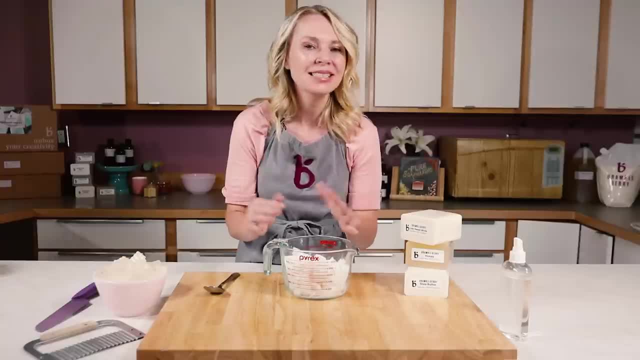 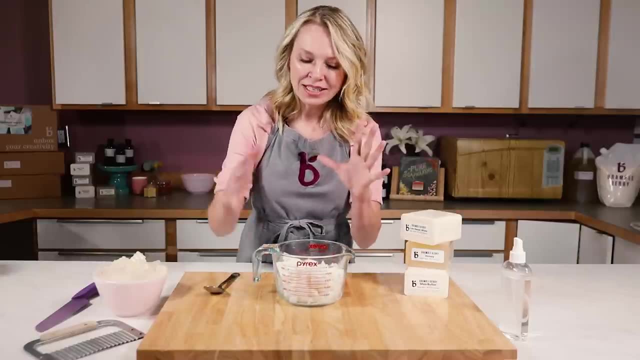 soap is not defective. it just takes probably about two, two and a half minutes at 30 second bursts in order to get your soap fully melted, and so i'm going to pop this back in for 30 seconds, check on it, and when it starts to melt, i like to give it a really quick. 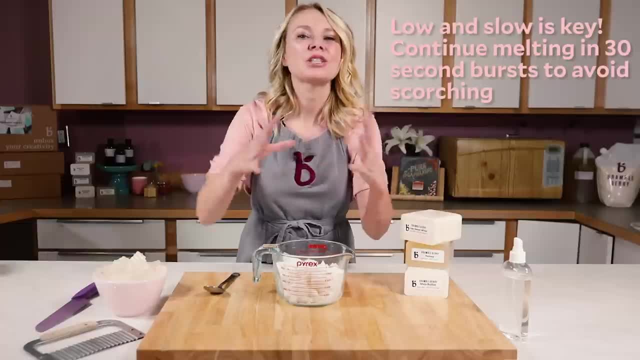 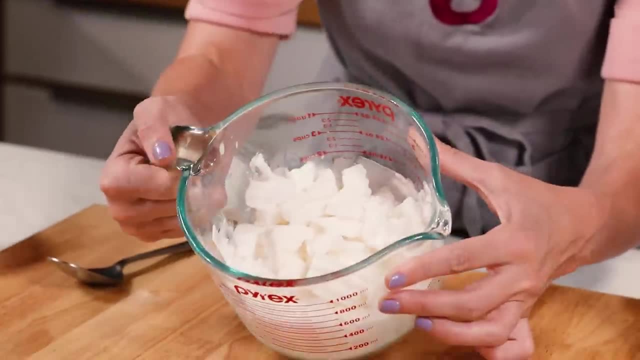 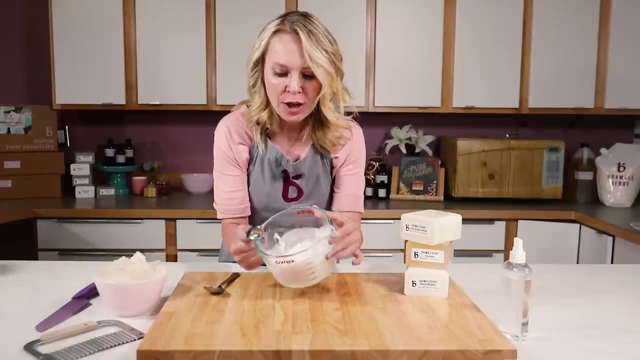 so that way there's not one single heat source that gets extra hot and potentially scorches just one part of the soap, and here we have 60 seconds of melting. so this is one pound of soap. you can see we've gotten a little bit more like meltage, to use the technical term. it still needs another minute. 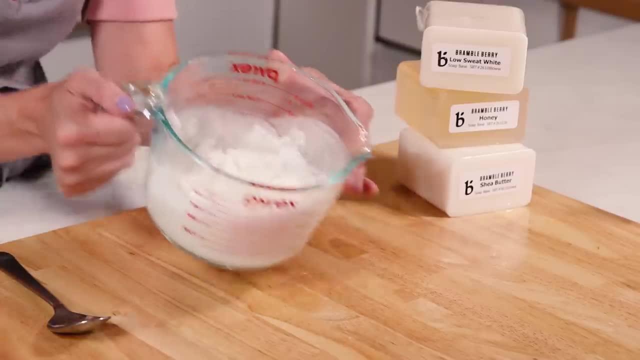 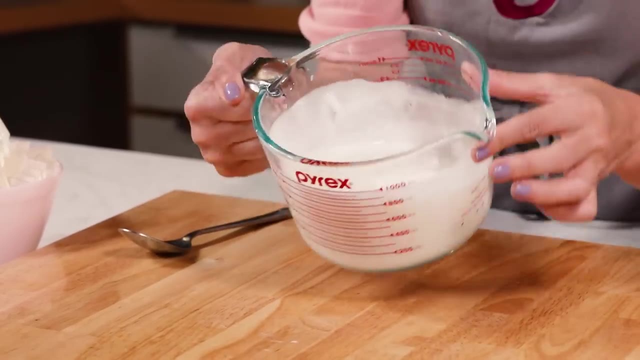 minute and a half for sure, so i'm just going to pop this back in for a 30 second burst. so this is one pound of soap at one minute and 30 seconds and you can see the meltage has definitely started occurring. now there are still a lot of chunks in here, so like big chunks, right? 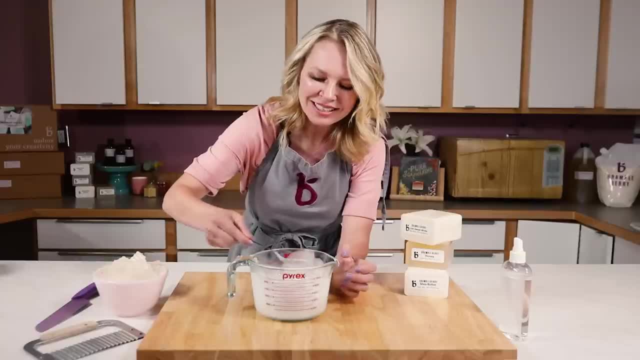 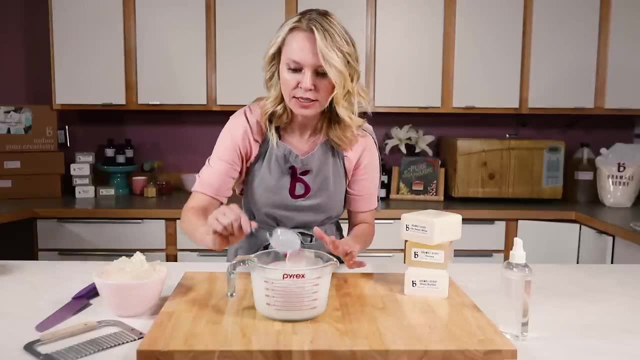 that's. this still needs another 30 seconds, so i'm gonna- and also i can tell this viscosity- it's too thick, so i'm just gonna go ahead and just kind of give this a really quick stir, make sure everything's mixed in evenly and put this in for another 30 seconds. 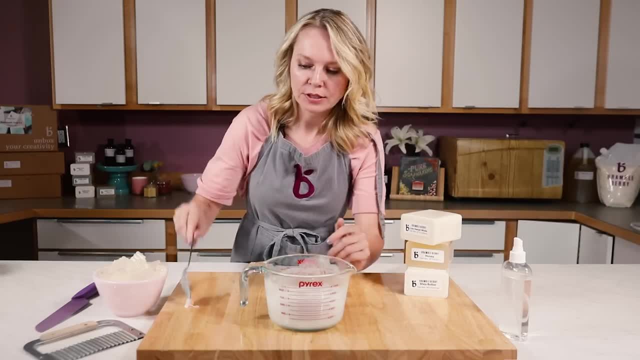 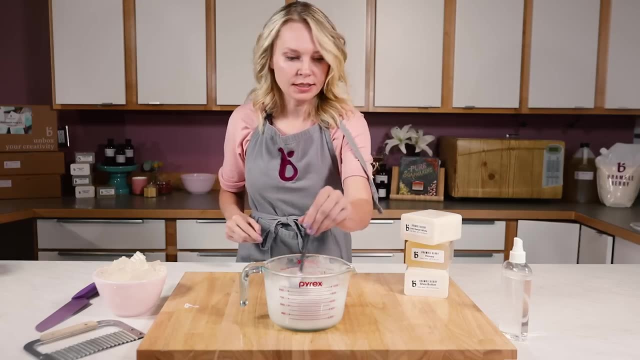 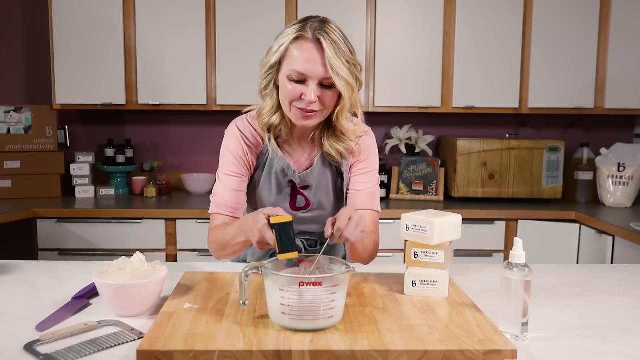 all right, we are at two minutes for this melt and pour soap and it is really perfectly melted. so this is a good viscosity and let me just check the temperature real quick. so you and i know what two minutes in my kind of standard microwave did. yours will vary because your microwave is. 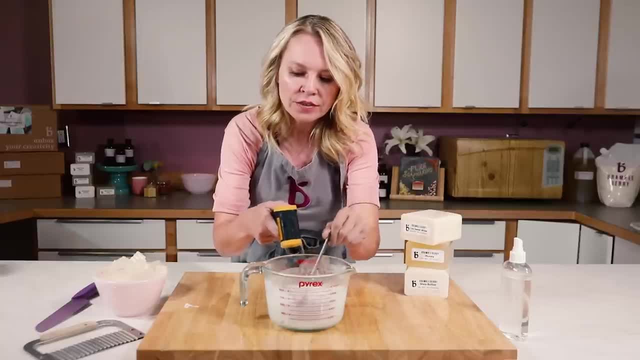 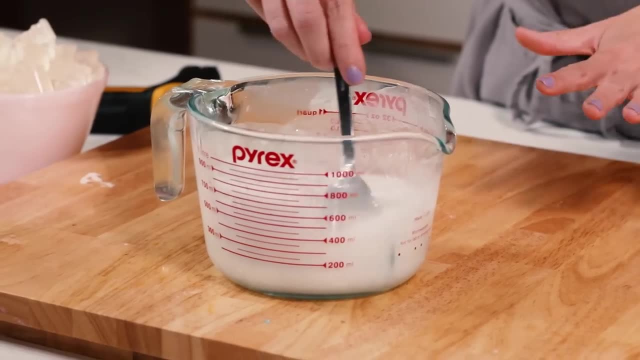 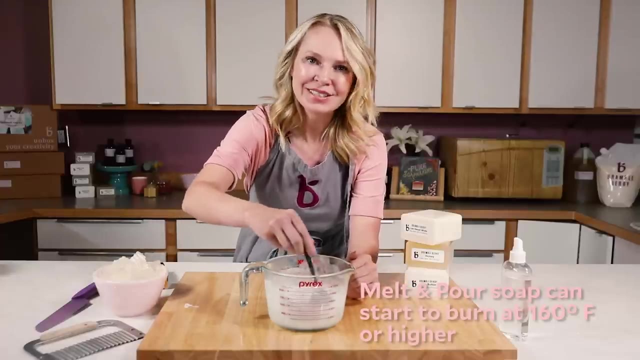 different than mine, but i'm at about 154- 156. so right there at the kind of top echelon of where i want to be. for meltage, you really don't want to let the soap base get over much about 160ish because it starts to burn boil and or steam, none of which is good. 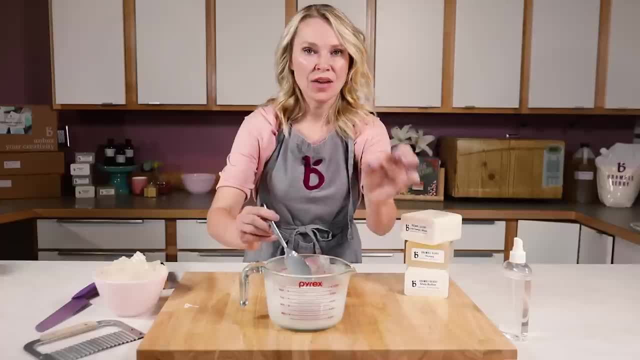 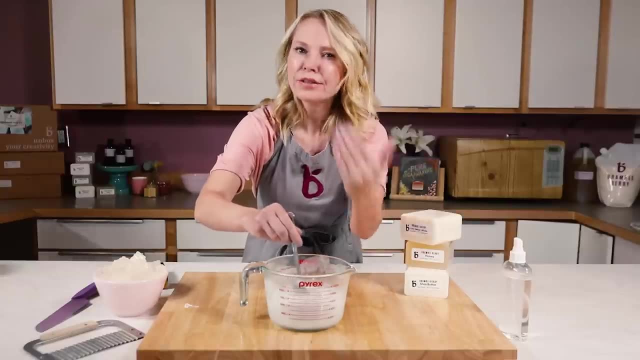 at this point, since i'm at like 156. if i was still to have any chunks in here, i would keep stirring and let the temperature of the warm soaps melt the last final bits of chunks, rather than trying to over melt or overheat the soap. so once your soap is melted, it's time to make it your own. 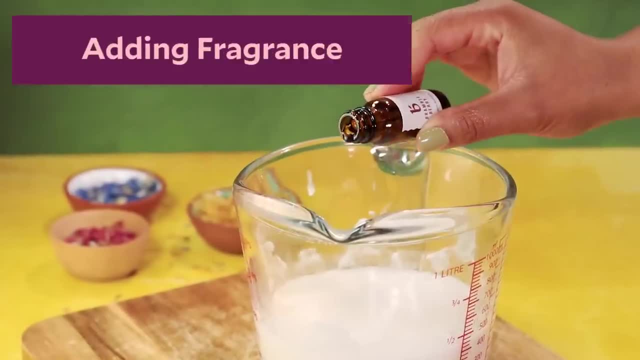 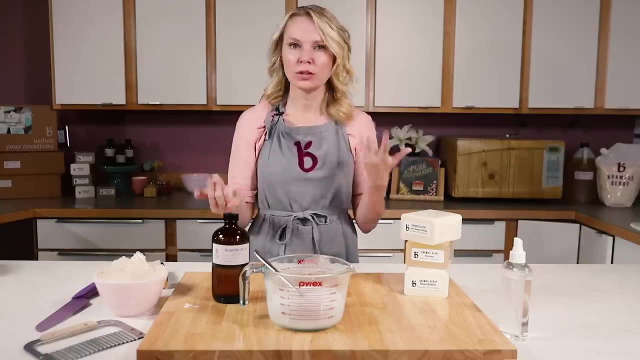 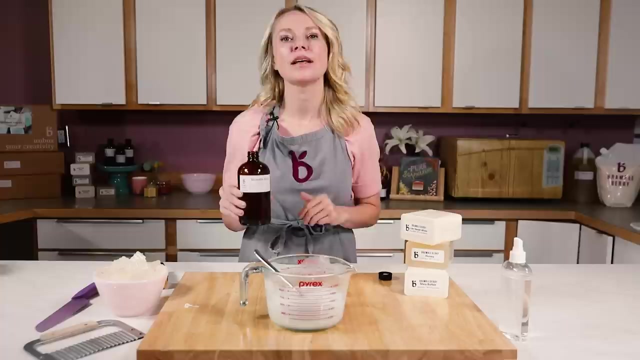 that involves choosing your color, your fragrance and your mold. you can use any skin safe fragrance oil and soap. so that means no candle and potpourri fragrances. but in this case, all of brambleberry's fragrance oils have been skin tested for safety and longevity and, of course, are phthalate free as well. once you've chosen the scent, you just 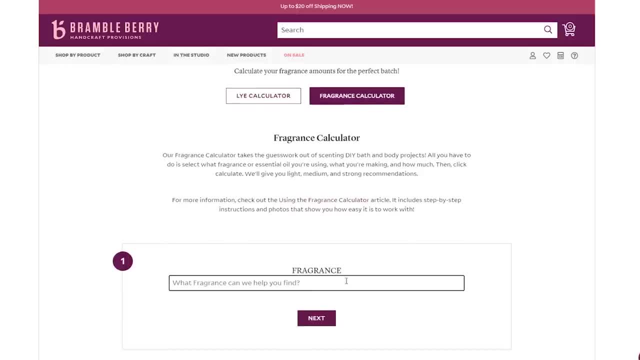 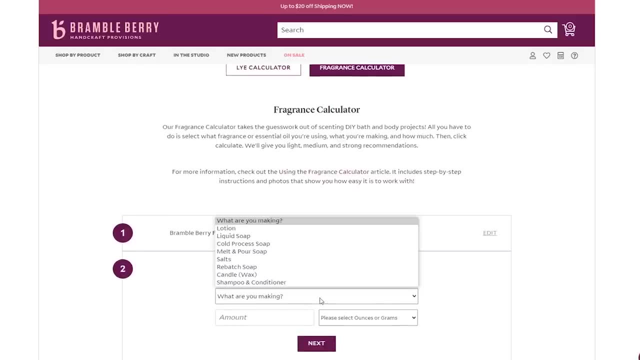 need to choose how much to use, and this is really easy with the brambleberry fragrance calculator at brambleberrycom. you simply choose melt and pour soap and enter how much soap you're making and then enter the fragrance oil. the calculator will give you a range of fragrance to use, depending on. 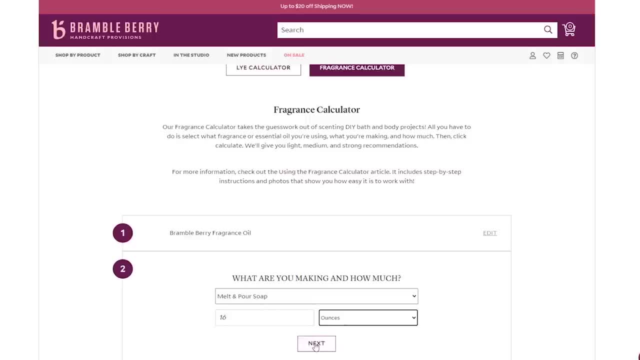 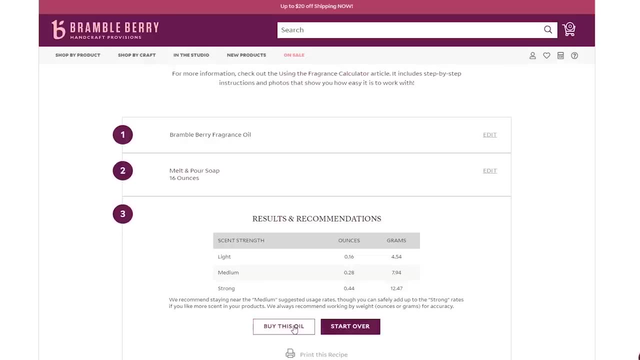 if you like light, medium or strong scents. if you're unsure, the medium choice is a very good the fragrance oil directly to your melted soap and stir in thoroughly. you don't want to see any oil streaks. so now that i know how much i need, i'm just going to go ahead and add that directly. 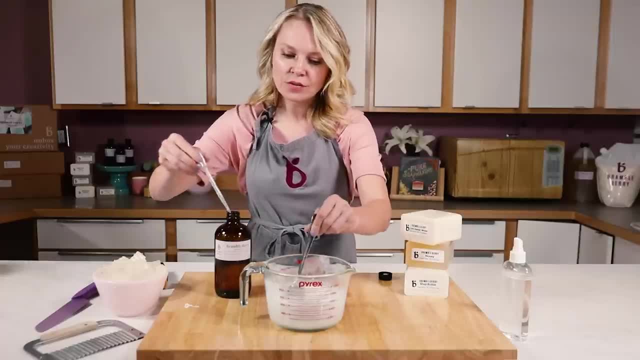 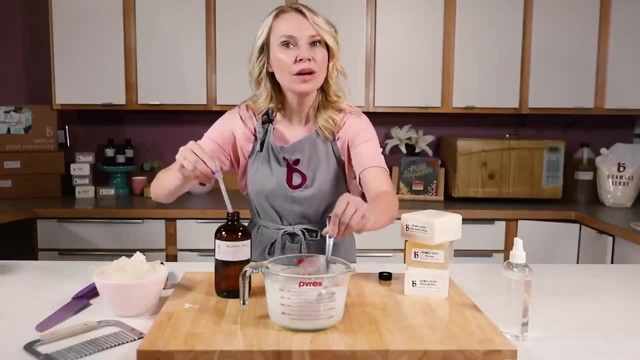 to my soap and i'm going to stir in really well. the thing is, if you're adding this to clear melt and pour soap you can see like: is the melt and pour soap still cloudy? does this need more stirring? but with white you never know. so be stirring for at least 30 seconds, because 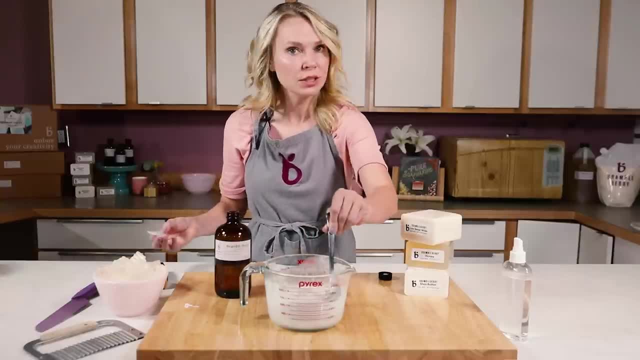 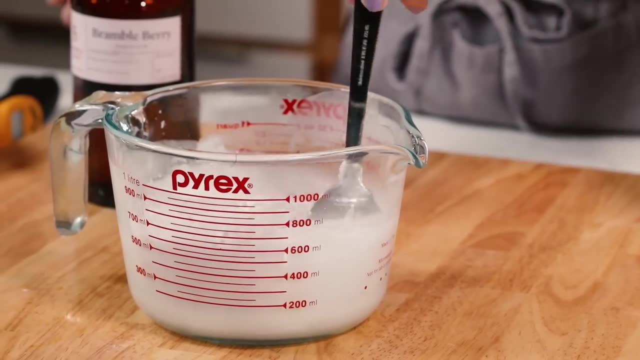 fragrance oil that isn't fully stirred into your soap can float to the surface of the the soap, or it can pit, meaning make weird little pits in your soap mold and ruin the soap mold. so stir longer than you think you need to for white melting for soap. 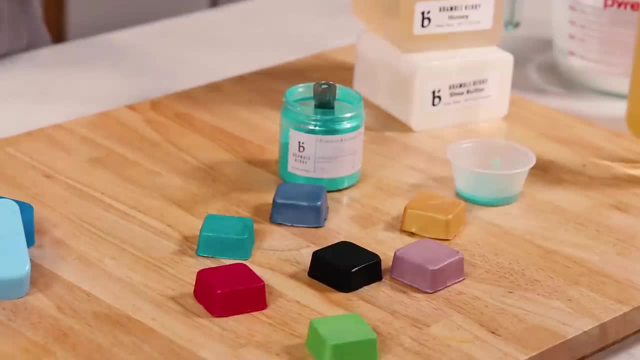 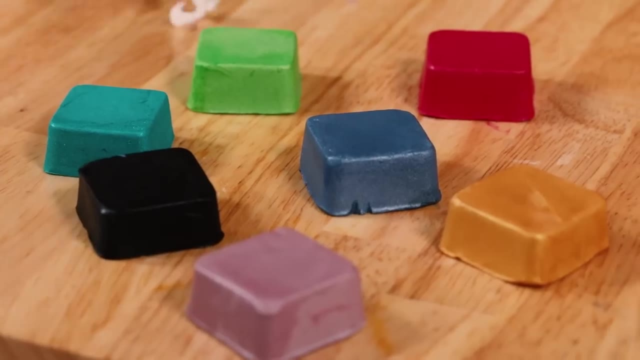 now let's talk about colorants for melt, and pour now. there's lots of colorants for melt and pour, but the two most popular ones are powders or dry colorants like micas or pigments and color blocks. powder colorants can be added directly to your soap, but they tend to be a little clumpy. 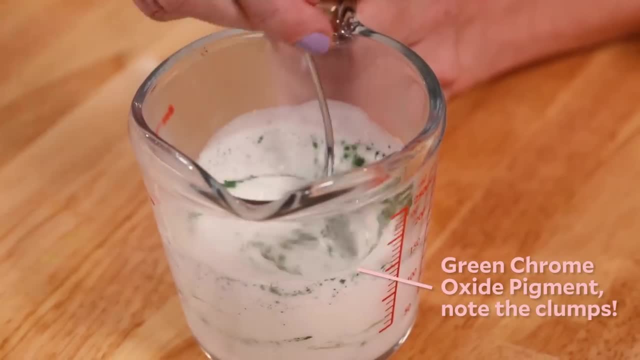 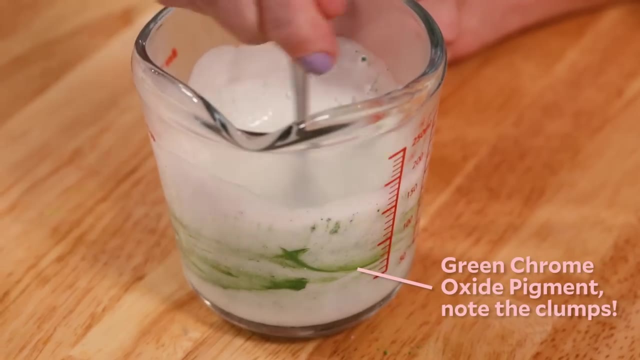 that's especially true for oxides and pigments which are heavier. i don't recommend dry pigments for melt and pour soap when you add them directly without any pre-mixing. now micas do mix a little bit better and then oxides dry, but dispersing those also makes it easier to disperse your dry. 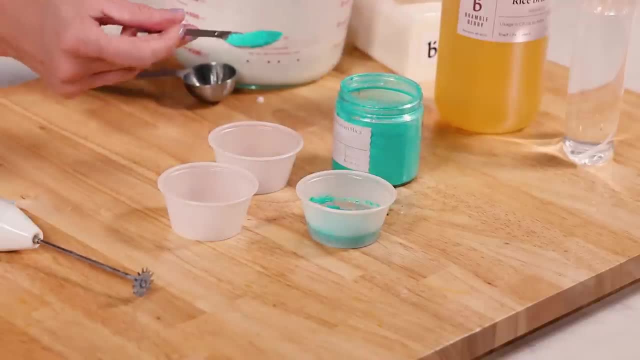 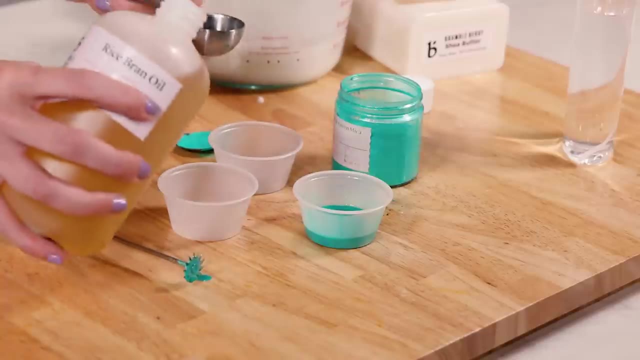 colorants. all you need to do is mix the powder into a liquid. isopropyl alcohol is a great choice for melt and pour because it does not affect the lather. but if you don't have that on hand, another option is to mix the powder with a small amount of a lightweight liquid oil. be careful with this. 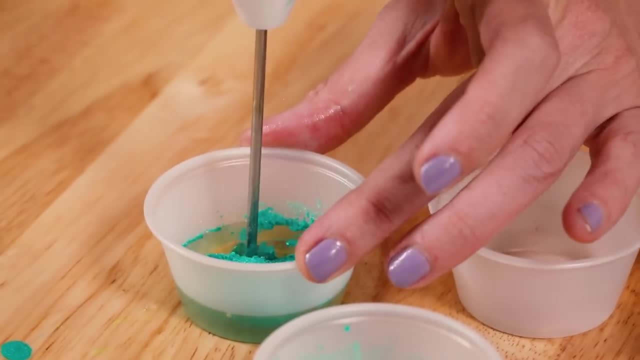 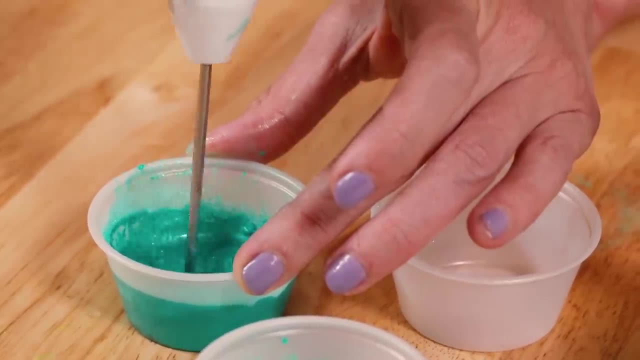 method, though, because it can cause a lot of dirts to the powder, and that's why i recommend you use a. has too much extra oil in melt and pour does affect or weigh down the soap lather. I recommend starting with one teaspoon of color to one tablespoon of alcohol or oil and adding the 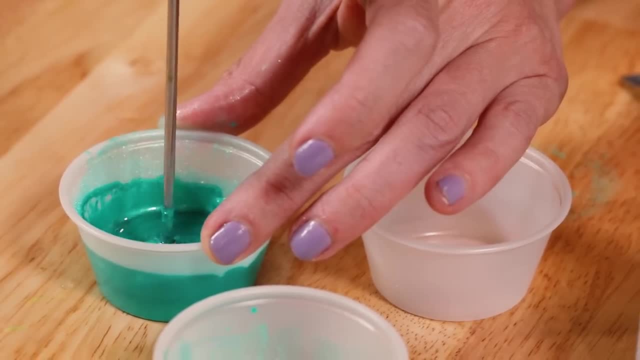 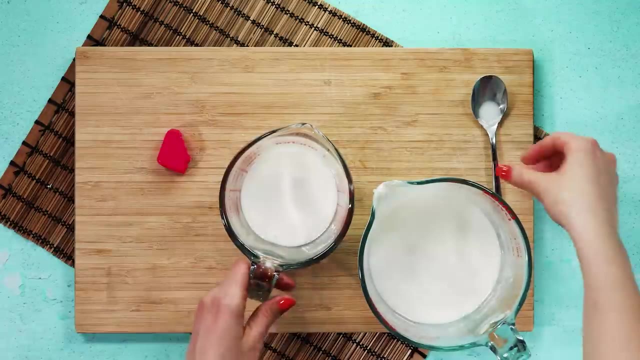 dispersed color to the melted soap until you're happy with the hue and shade. Another option, which is my preferred method of adding colorant to melt and pour soap is to use color blocks. Color blocks are exclusive to Bramble Berry and are created in our lab in Bellingham, Washington. They're 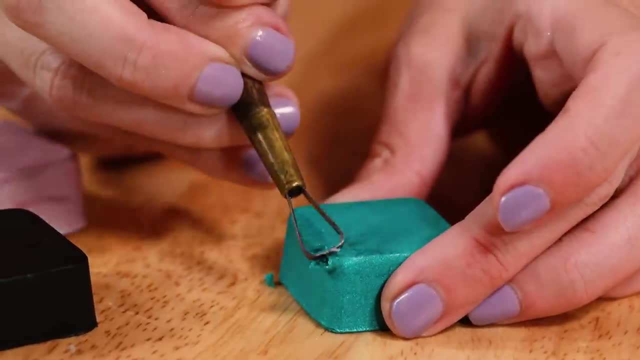 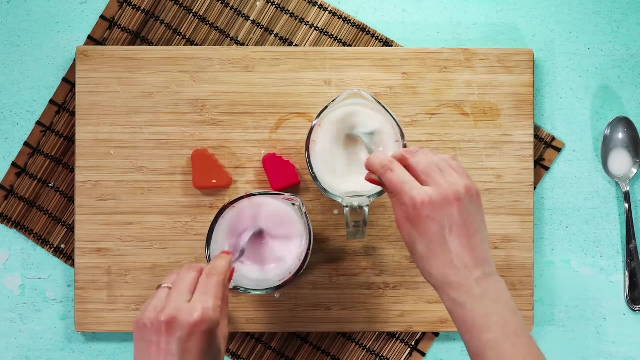 highly concentrated colorants that are pre-mixed into melt and pour soap. so all you have to do is add shavings or chunks of this color block to your melted soap and stir. The heat will melt the blocks and disperse the colorant throughout your bar of soap. In addition to these types of 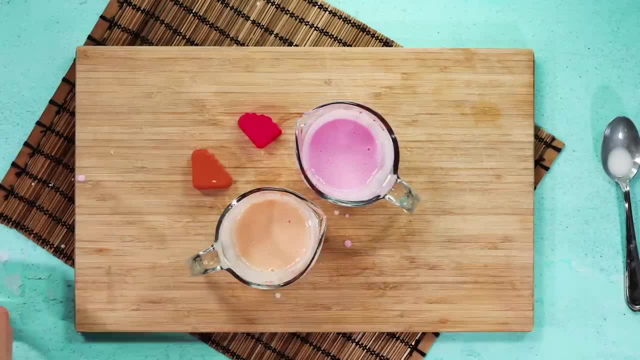 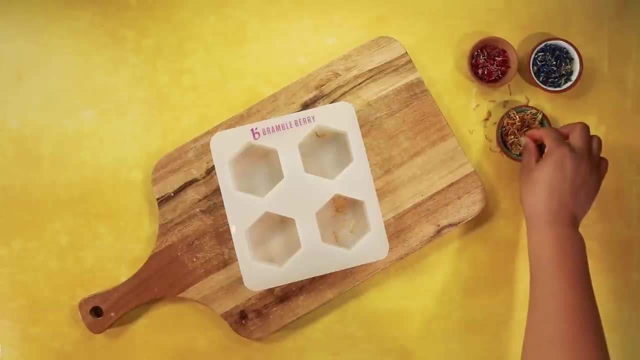 colorants. it's also fun to work with natural colorants in melt and pour soap, such as activated charcoal, clays, turmeric and more. Check out our melt and pour playlist for more ideas and recipes on using natural ingredients. Botanicals and exfoliants also work great in melt and pour soap. 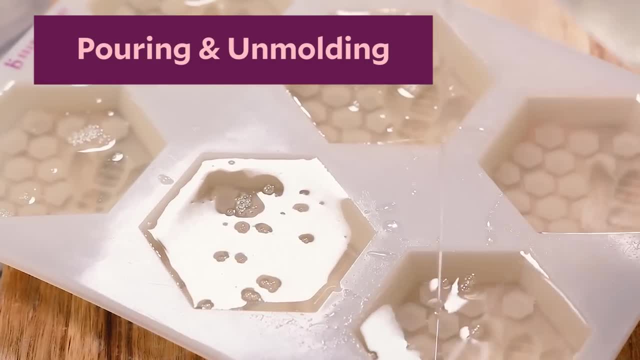 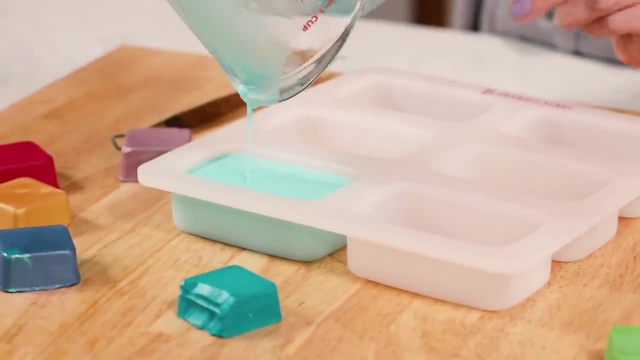 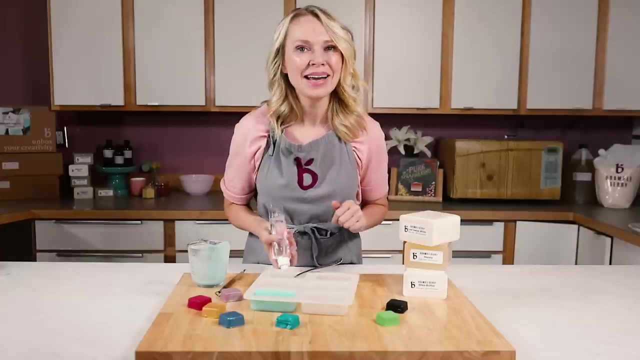 Once you're happy with your color and your fragrance, it's time to pour into the soap mold And I see just a couple bubbles forming at the surface. so I'm just gonna take a little bit of isopropyl rubbing alcohol and spritz and those bubbles will go away. So, obviously, having a little 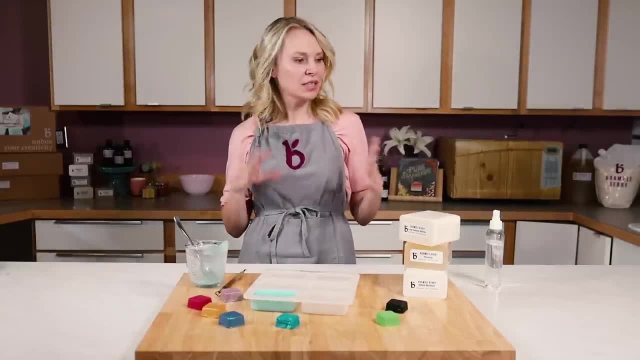 bit of bubbles on the back of your soap, not a big deal, totally aesthetic, it's just a nice finishing touch. Now, what doesn't work is like water. Water doesn't work to get rid of the bubbles and you can go all the way down to 91%. So I'm just gonna take a little bit of water and I'm just gonna take a. 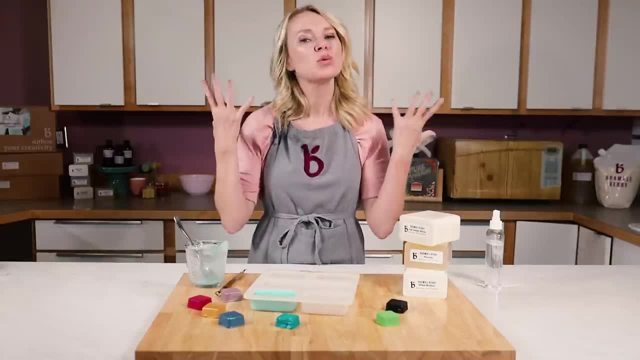 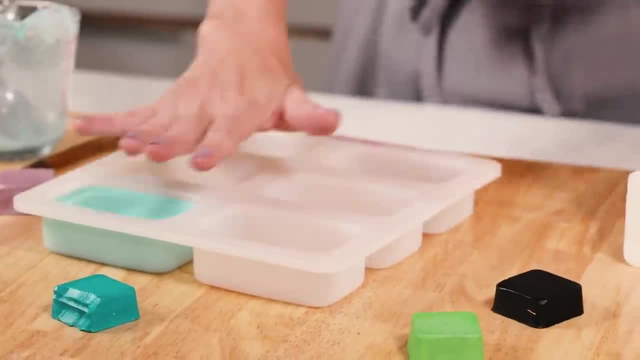 little bit of soap, and I'm just gonna take a little bit of soap and I'm just gonna take a little bit of rubbing alcohol and still have the bubbles pop, because what the alcohol does is it breaks up the surface tension of the bubbles, which is what allows those bubbles to pop, and then give you 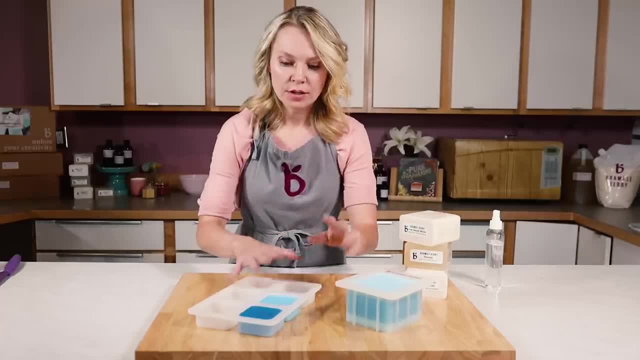 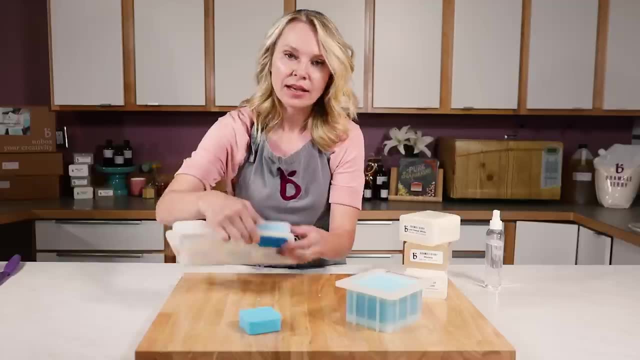 a smooth, even finish on the back of your soap. Once your soap is hardened in the molds, it's time to remove the soap. And now, how long that takes to harden in the molds depends on the size of your mold. So, like little guys like this, it's about two to three hours to harden, but like loaf. 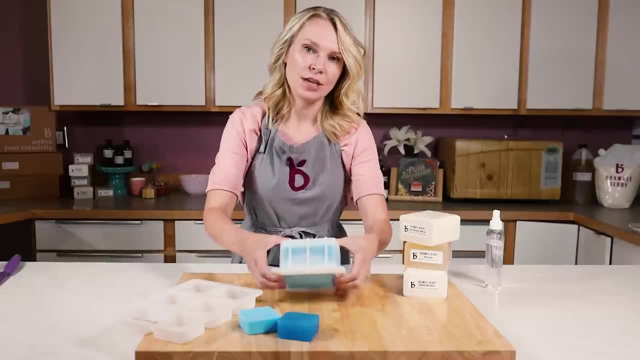 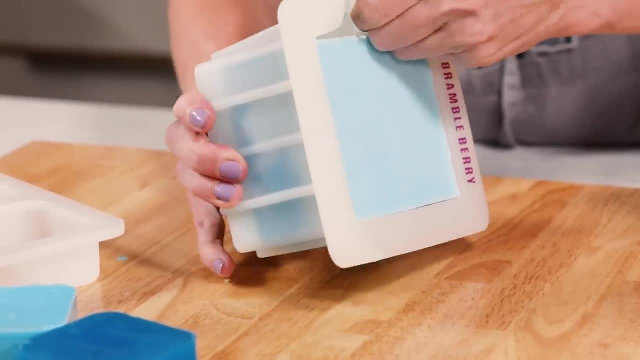 molds well, they can be five to six hours And you always want to make sure that you're using, always want to make sure that your soap is fully, absolutely hard before you try to release it. otherwise it can leak or be too soft and ruin the design, which is never fun, And sometimes the loaf. 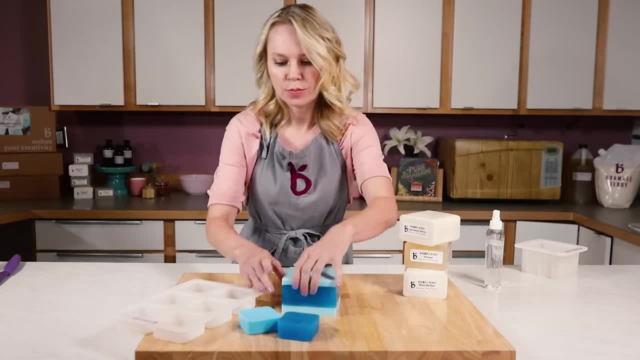 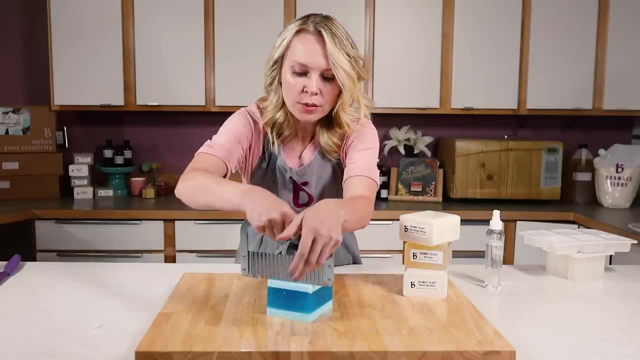 molds. just take a little bit of elbow grease. They're totally worth it, because you have such beautiful, even lines that are nice and shiny. Chopping into your loaf soap is really easy. You want to make sure that you're using a very sharp knife, however, so I'm using the Bramble Berry Crinkle. 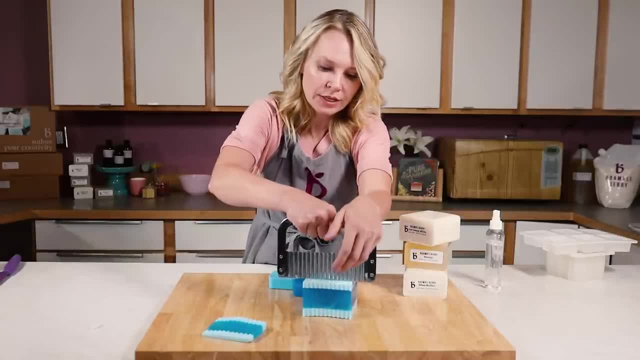 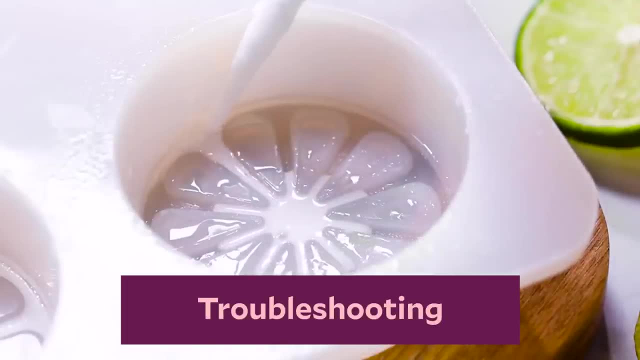 Cutter just to give it a little bit of a sharp cut, And then I'm just going to take a little bit of to give it a little bit of interest. I think it looks beautiful and it smells delicious. So let's talk about some troubleshooting things that can happen At this moment. our soap has been 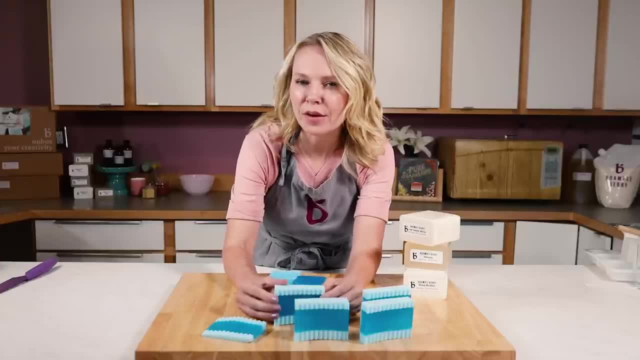 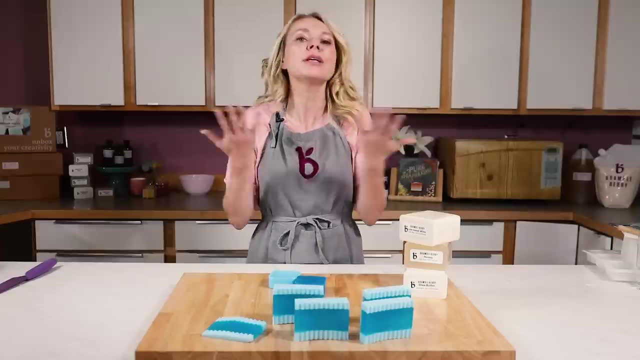 released from the molds. It's gorgeous. You might come back the next day, though, and find little tiny droplets of something we call it glycerin dew on the soap. What's going on, and how do you solve it? So it's literally called glycerin dew. Melt and pour. soap has added glycerin, which is a 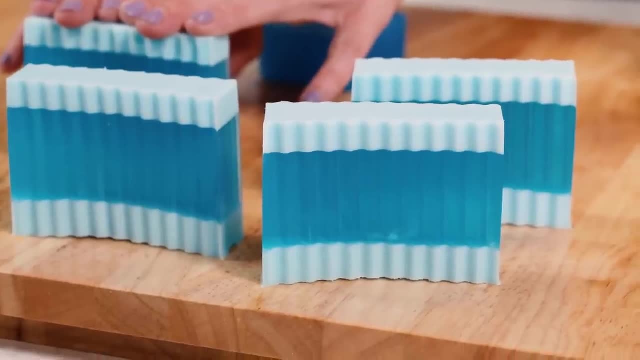 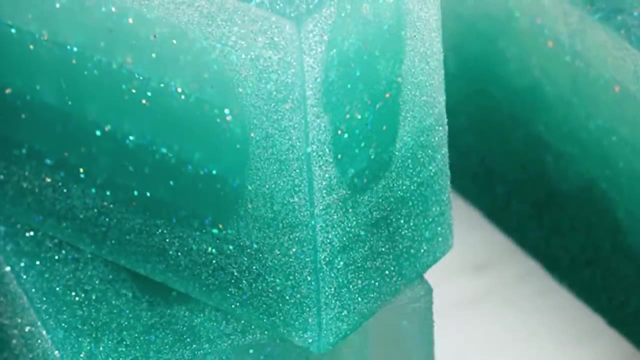 pigment that draws moisture to the skin. It also helps the soap re-melt down easily. It also, though, can draw moisture from the air and sit on top of your soap, So if you're in a humid climate, you might come and see all this dew on your soap and go. what do I do? It's really easy to solve that. 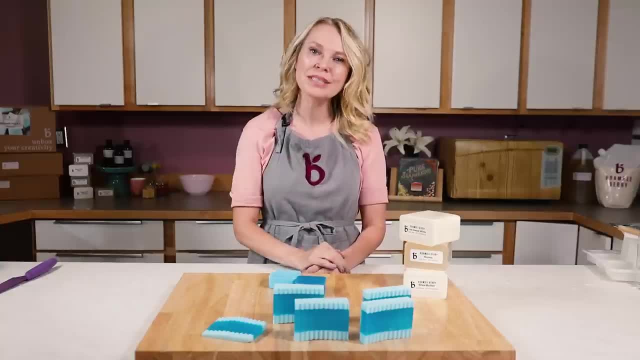 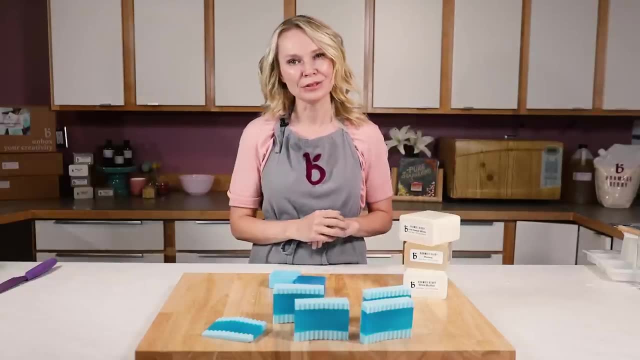 All you do is run a fan over the soap right after you pull the soap out of the molds and let that happen for about 12 hours, and that wicks all that moisture away and keeps your soap fresh just like it came out of the mold. Or another option is just to simply use low sweat like cold process melt and 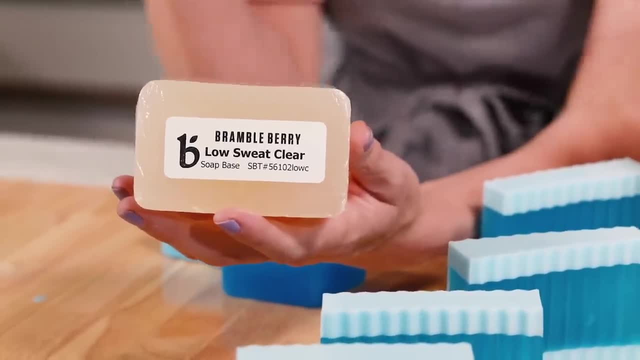 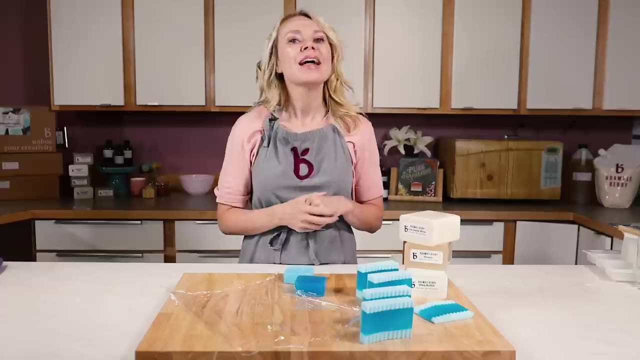 pour soap. What that means is it has less liquid glycerin added during the soap making process, so it's less prone to forming glycerin dew. Also, it's a little harder coming right out of the soap mold. Last but not least is how do you wrap your soap? Well, honestly, you can just use regular old saran. 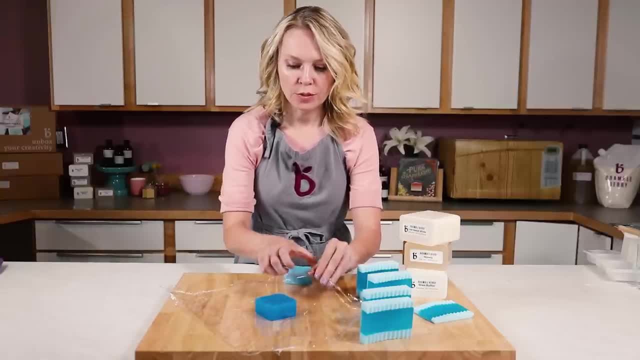 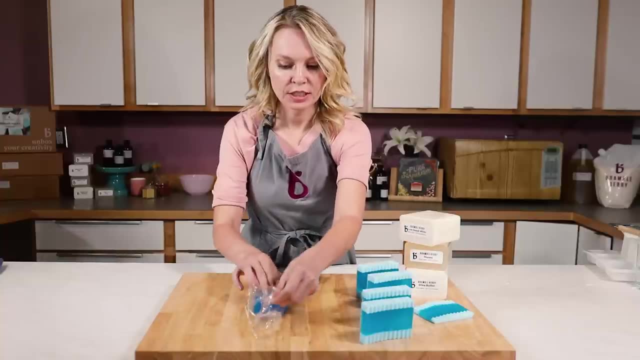 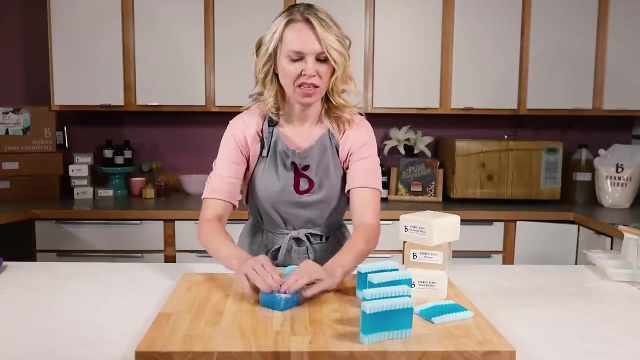 wrap, and so the way you do that, it's pretty easy. You take the bar of soap, you put it face down and pull here. The whole key is, you want it to be pretty tight, and so what I like to do is just pull tightly here, pull tightly here, and then there's this big, huge at the back. so I just 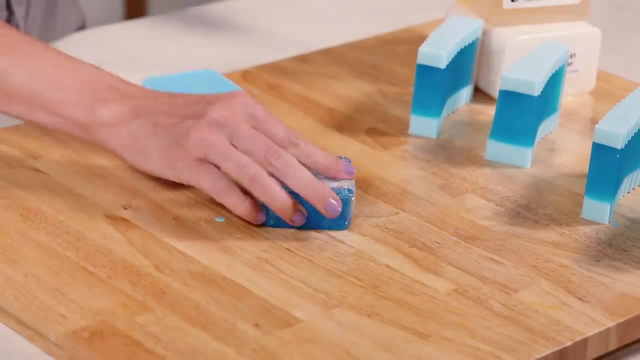 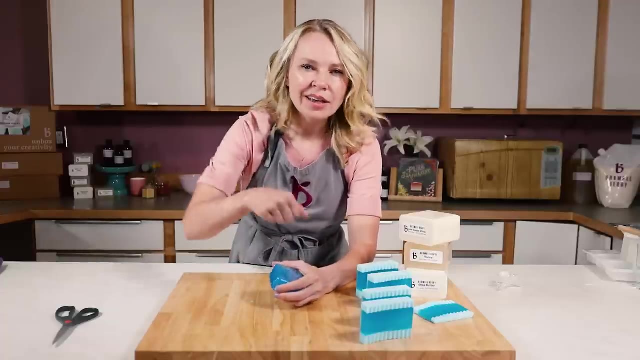 take some scissors, kind of do this, and then you're either totally wrapped right now, like this is wrapped, or and then you can just put a label right there. Some people like to do just a little bit extra with like a heat gun or something, just to really shrink it on there, especially if you have. 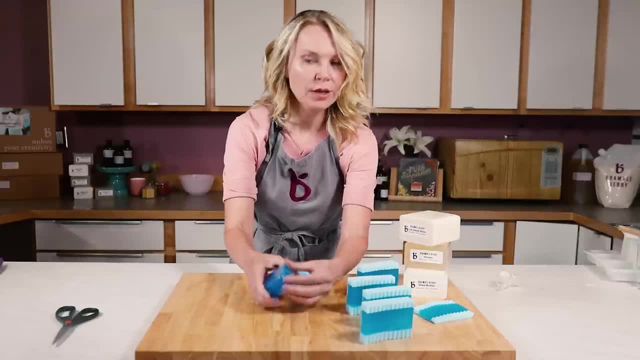 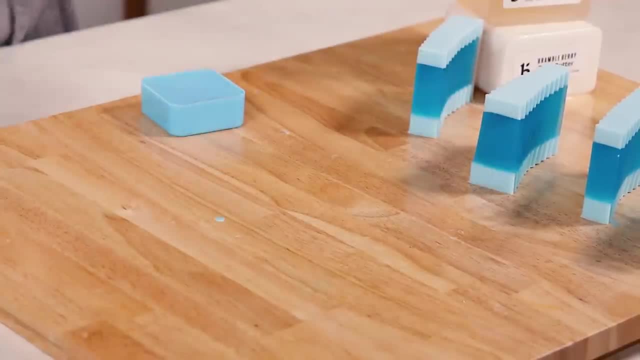 something that has like a design on it. But in this case you're wrapped up, you're ready to go, you can give this away, Use it right away, sell it right away. again. it's melt and pour soap. no cure time, no drying time. Once your soap is wrapped, your soap will not get glycerin dew and it's going to stay fresh. 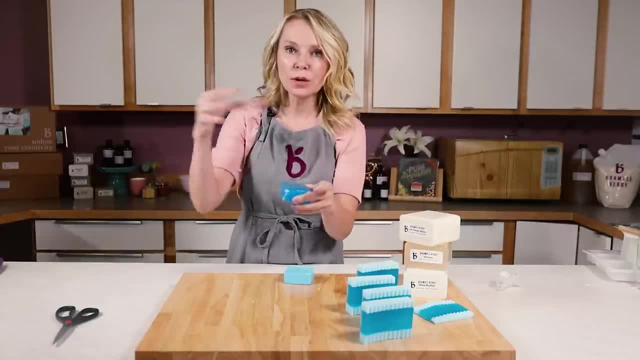 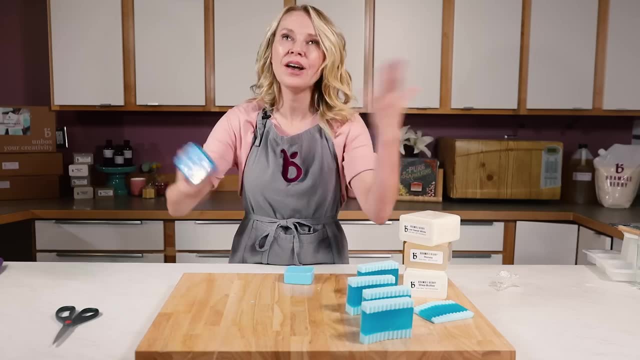 and clean and of course, the reason it doesn't get glycerin dew is this is preventing moisture from entering the bar of soap right. there's a barrier here, so it helps little sticky fingers in case it's on a store shelf and it also helps humidity from not forming on the bar of soap. One of the 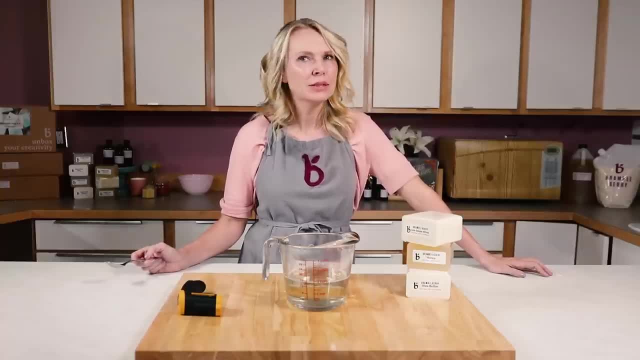 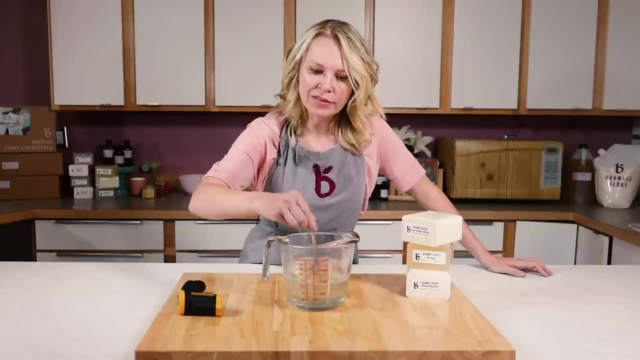 most beautiful things about melt and pour soap is it's really hard to mess up. One of the surefire ways to mess it up is to overheat it. In this case, I intentionally overheated this soap to about 207-211 degrees, and I mean there is steam rising from it even. 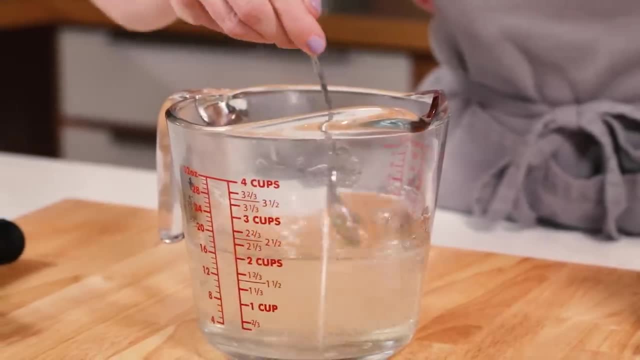 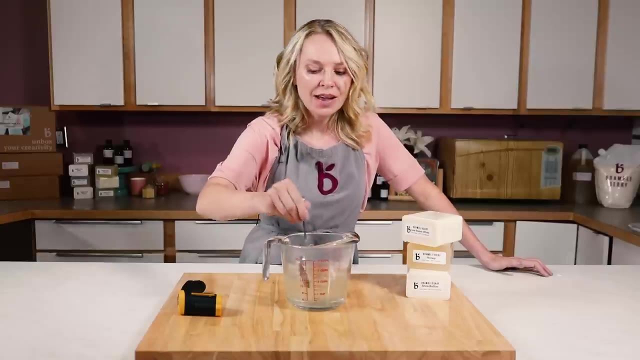 if the camera is not catching it. So what happens when you overheat your soap? Well, you can change the color. In this case it didn't change the color all that much because I didn't overheat it that much, But really the texture changes a lot and it gets gloopy and then it hardens. all weird when. 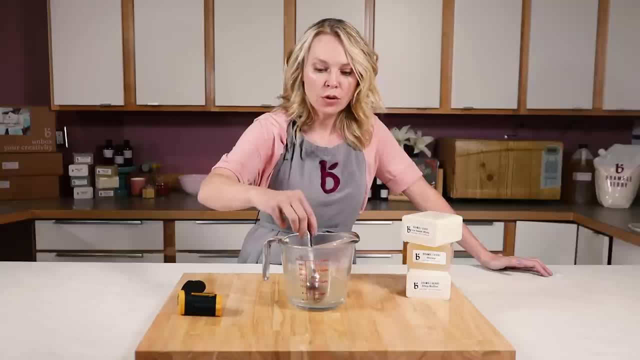 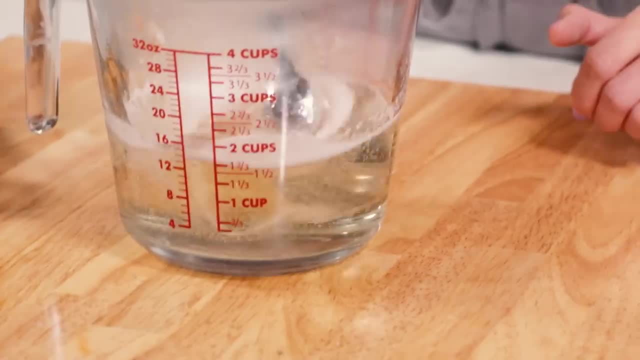 making the soap And so it's going to change the texture of the soap when you're pouring it and any potential design possibilities. And, like I said, if you overheat it a lot it goes really yellow. So when the soap overheats it is really hard to get really technical, detailed soap. So 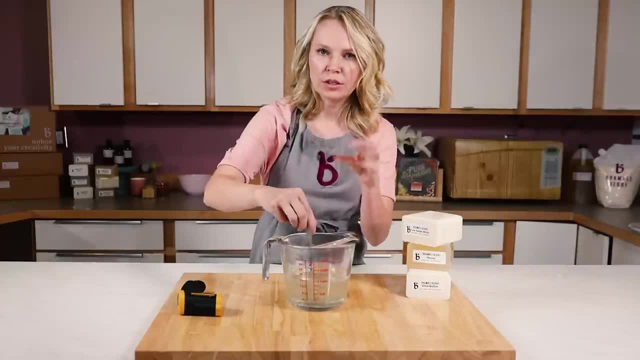 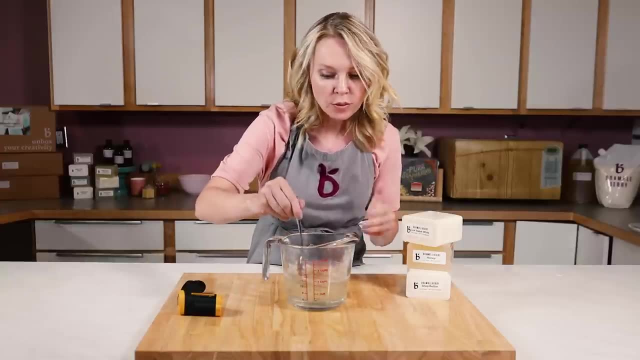 swirls and think of like really cute technical looking soap molds, because this is really. it turns kind of snotty, like it's really thick and really gloopy and not great. So you always want to make sure that you're maintaining your temperature at 160 and below when using melt and 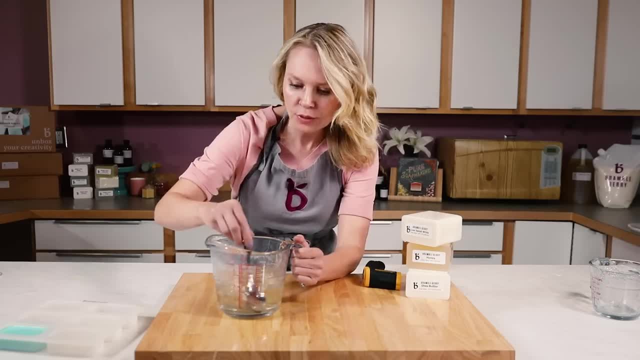 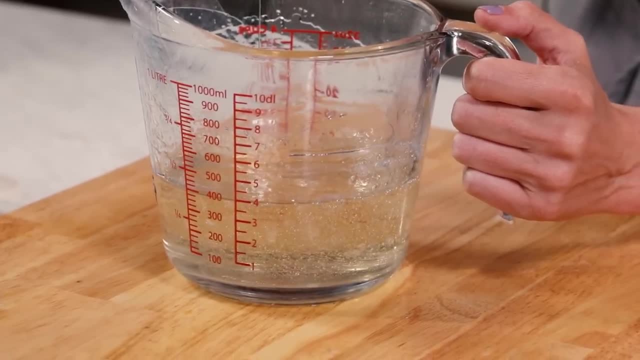 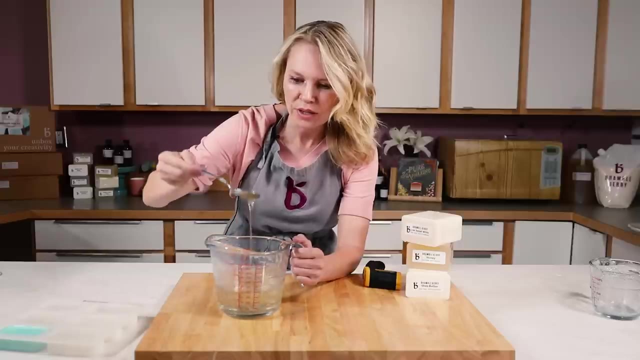 pour soap. So this is my boiled soap And I hope you can see it is a little bit gloopy. It's just like this weird kind of snot. there's no chance it's ever going to get any sort of great details in there, And it's just it gets clumpy and kind of starts to harden up really fast. So it's still. 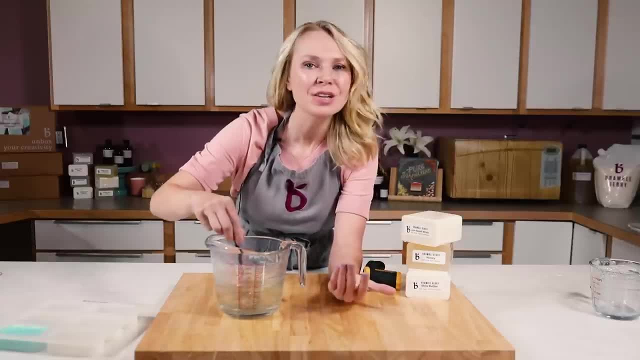 so not all hope is lost. it's still going to lather, it's just not going to look exactly how you want it to look And it's not going to get to the design qualities you want. So temperature check, this is literally. 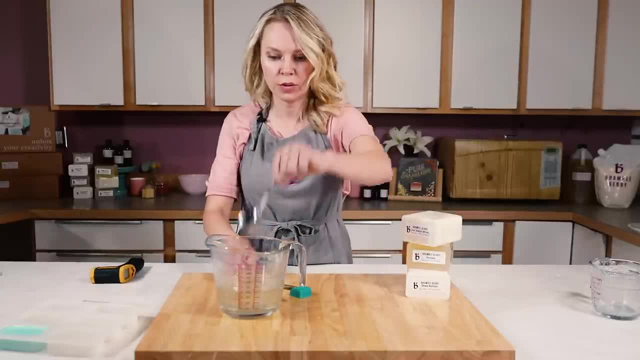 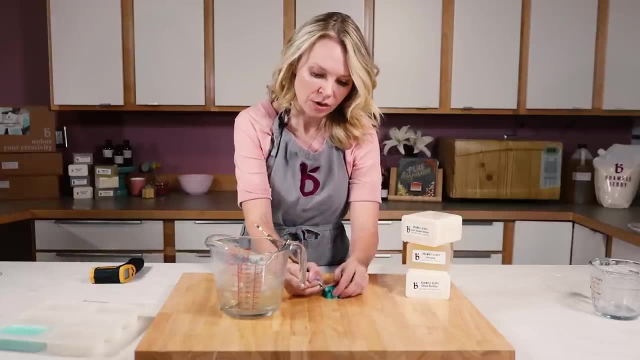 at exactly 140.. And this should be really fluid and gorgeous right now at this, And it should be the perfect time to add colorant. but it is definitely not going to be, because it's not going to melt my colorant And it's also not going to pour cleanly and easily. I mean, this is just 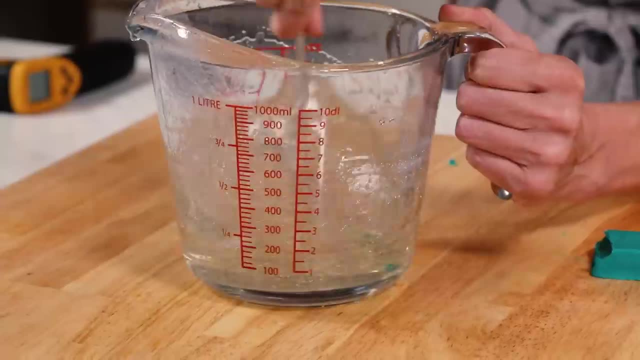 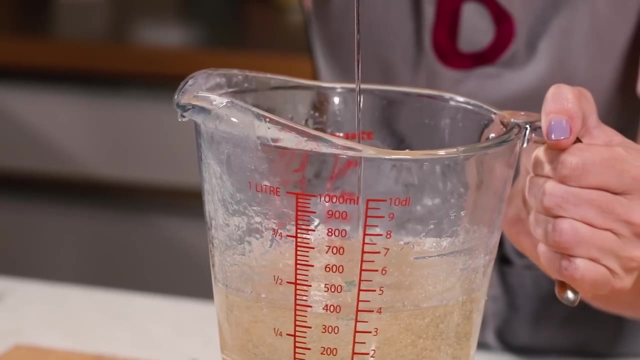 this is not. this is not great. So moral of the story: definitely don't overheat your soap. it's still going to be soap, but you're never going to get what you want out of it, Because this is, this is just not, is not working Okay, so now I'm going to try. 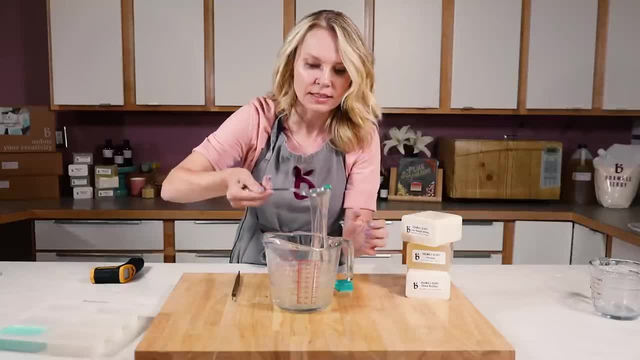 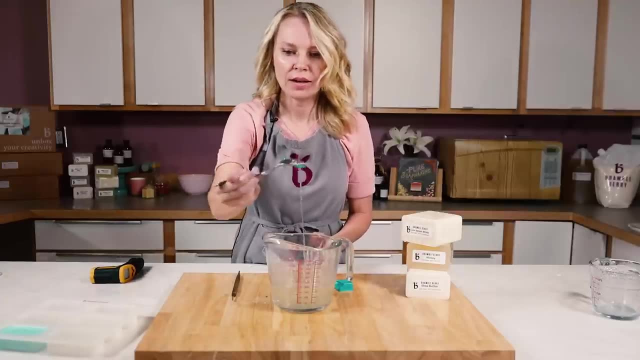 and get this color block out of here, because it's clearly not going to melt And if I let that stay in my soap it's just going to be this crazy, insane sort of block of color. I'm gonna do that And I'm just going to let this sit right here and try and get this poured into some soap molds, just. 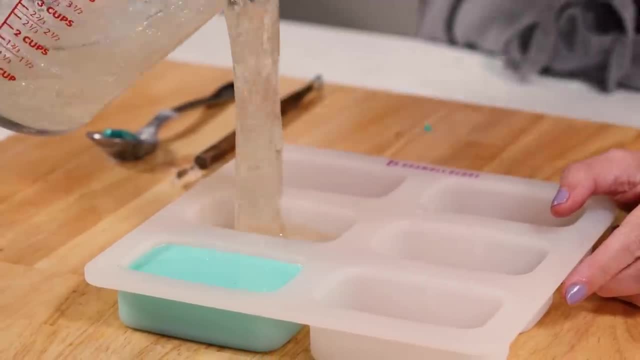 so I have at least a little bit Oh of actual soap, because I don't want it to totally be ruined. But yeah, this is, this isn't going to get. it's going to become like this. I'm going to leave it for a 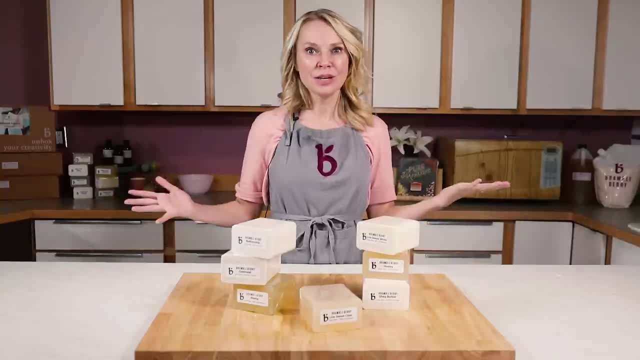 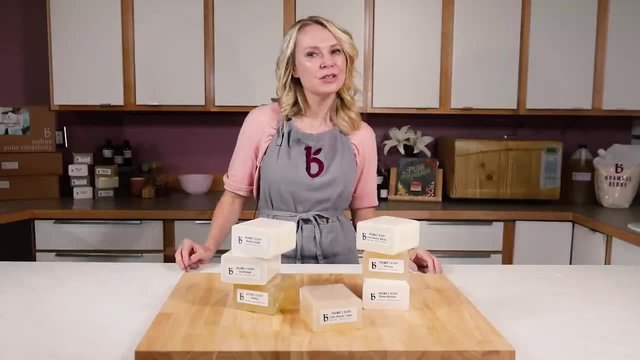 great thanks so much for watching today's episode on the basics of melt and pour soap making. if you like this video, give it a thumbs up below and, of course, if you're not subscribed to this channel, subscribe to the channel so you're notified every single time we come out with a brand new video. if